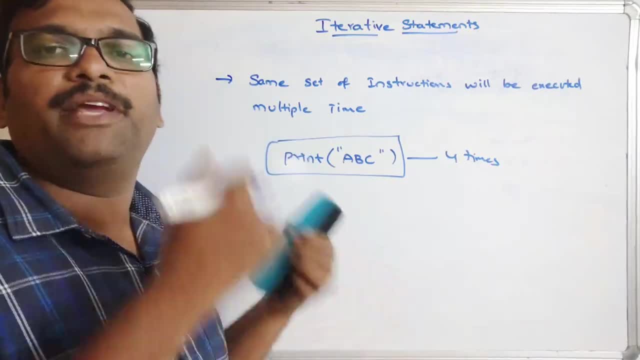 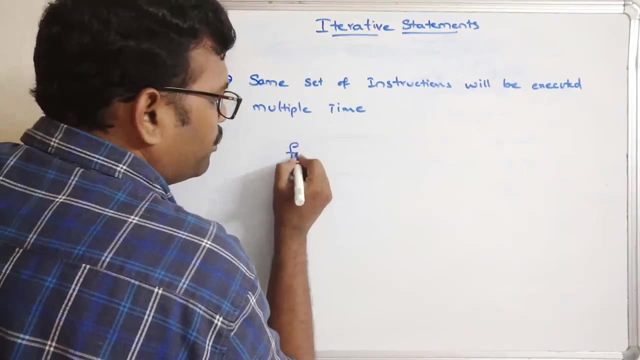 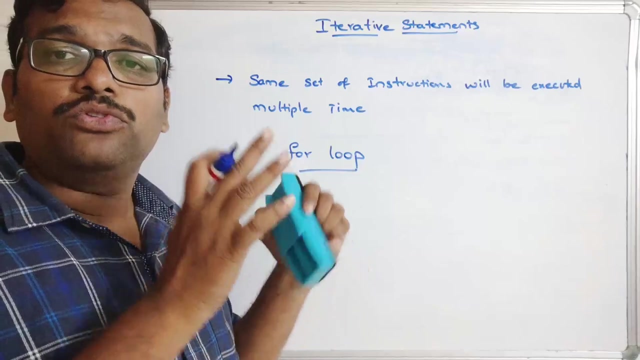 times. We have to write only once, and the same instruction will be get executed multiple times, And for that we are going to use one iterative statement called for loop. We call it as a loops, So the first one is a for loop. So here the question is where to stop. 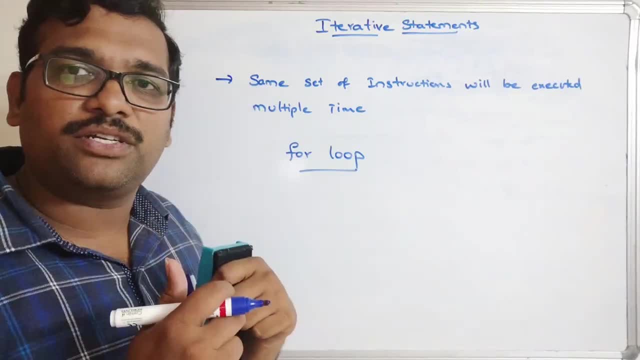 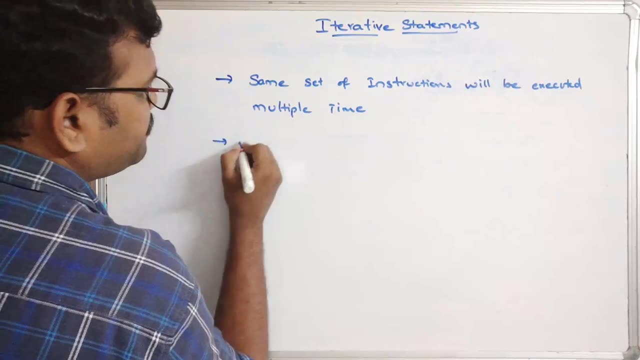 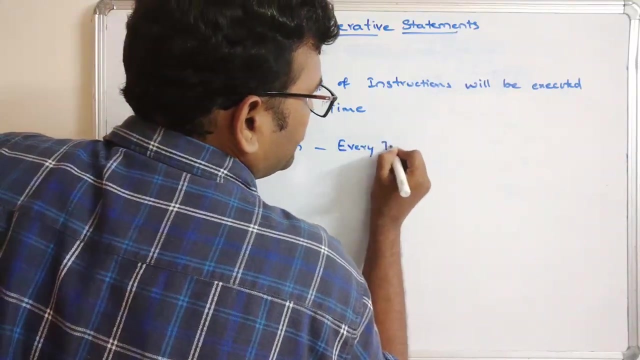 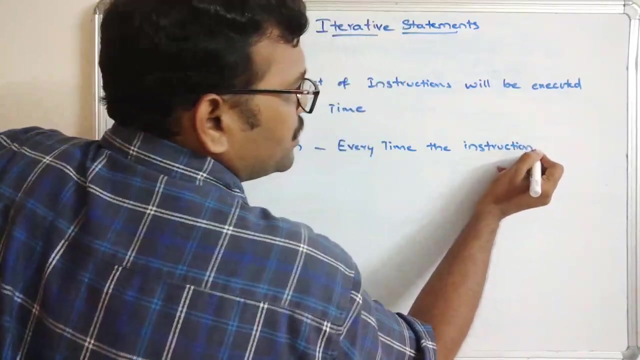 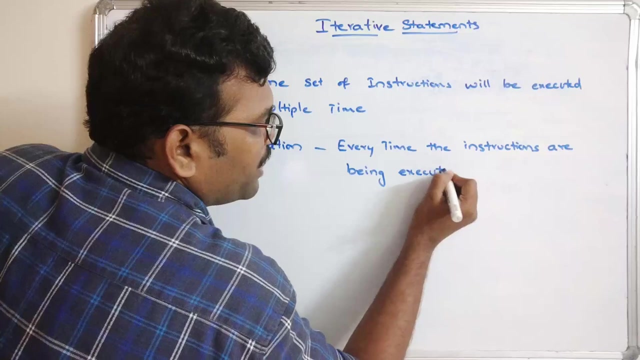 the iterations. So every time the set of instructions are being executed is called an iteration right. So I will write here iteration, Iteration. iteration means every time the instructions are being executed, Instructions are being executed. So, for example, if one instruction is being executed four times, we call it as a loop, Right, So this is called a loop. Alright, let us here, for example, if all instructions are being executed multiple times. now, what I am going to do is say I call it as a loop. I can set the version of repetitions. This: 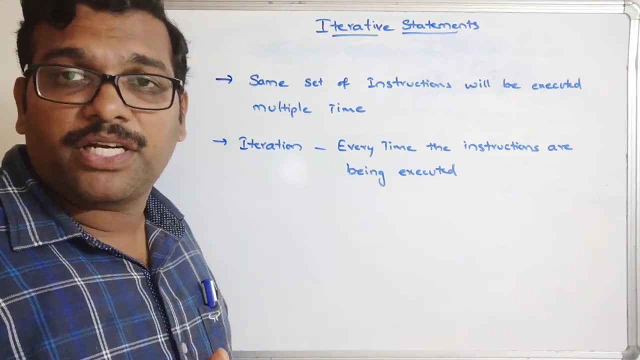 is second extension running. that is firstешst, and then I call it as a loop. Only I could be able to change an existing one very quickly. if we start with this as partially, we cannot four iterations. If the same instruction is being executed for 10 times, we should call it as a 10. 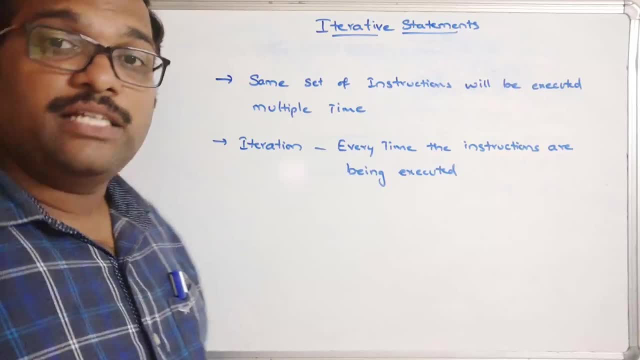 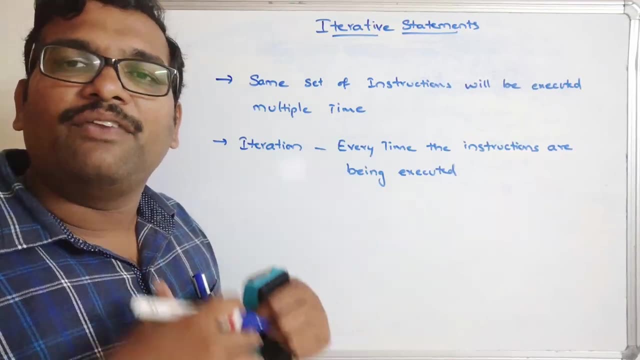 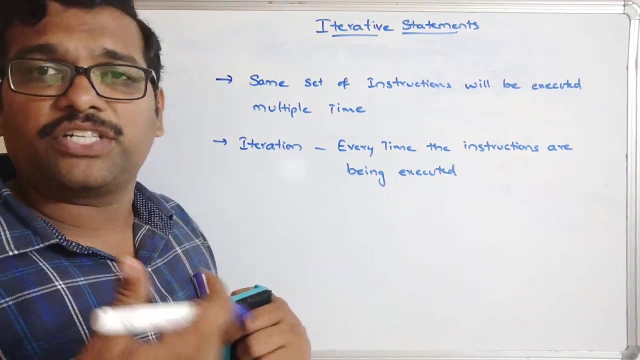 iterations. So here the question is where to stop these iterations. So if you are not able to stop these iterations, what happens? It will lead to the infinite loop, So multiple times. it will be keep on executing the same set of instructions infinite times. So we should be very careful. 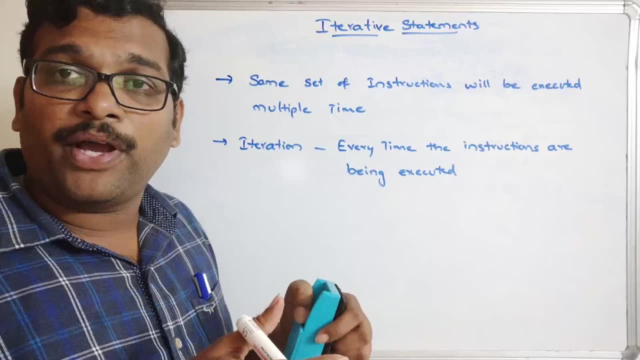 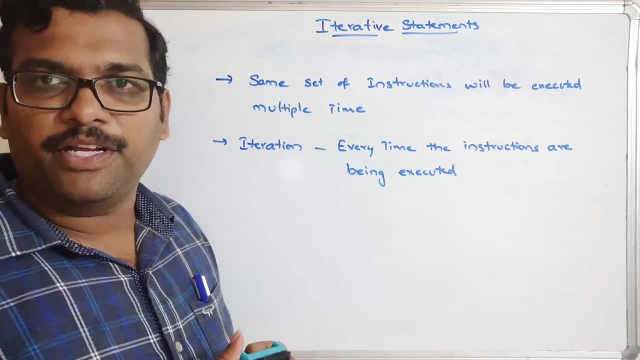 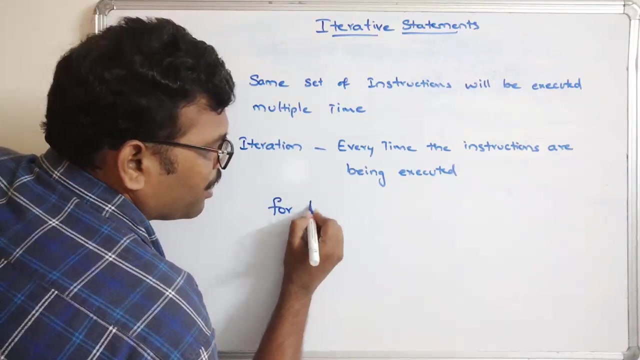 while writing these iterative statements, because after some finite number of iterations, so the loop should be terminated, The control should exit its termination right. So one such iterative statement, we call it as a for loop. for loop, right For loop. So here: 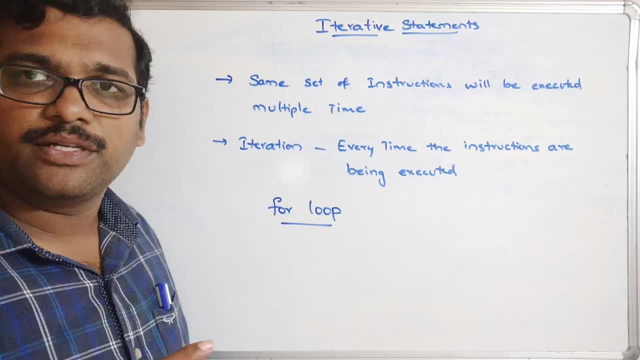 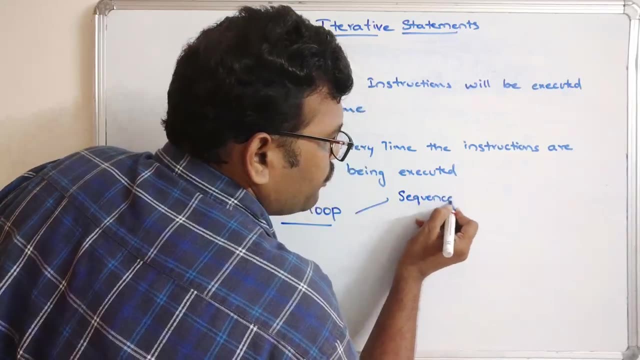 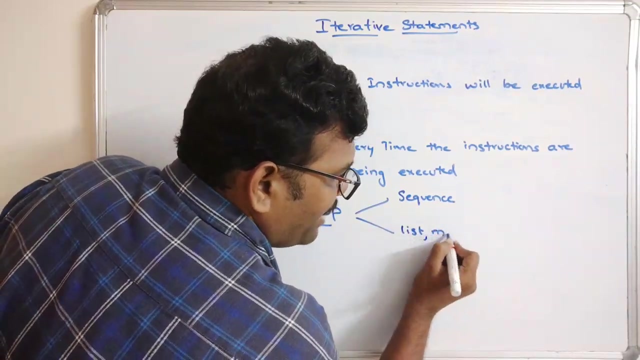 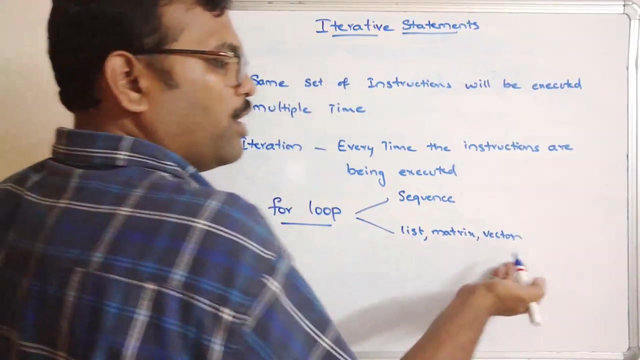 the for loop can be implemented in two different ways. So one is by using a sequence- a sequence, and another one by using the data structures, like a list or matrix or a vector right. So we can use any one of these three data structures or, directly, we can use the. 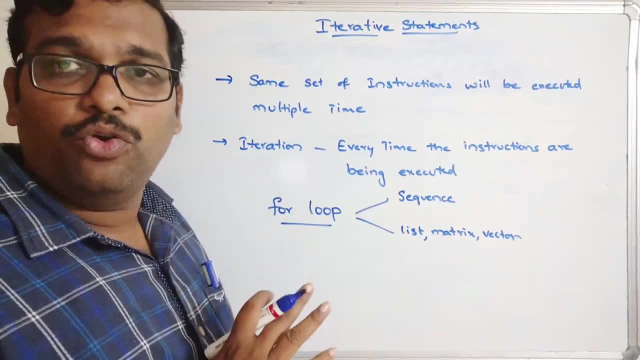 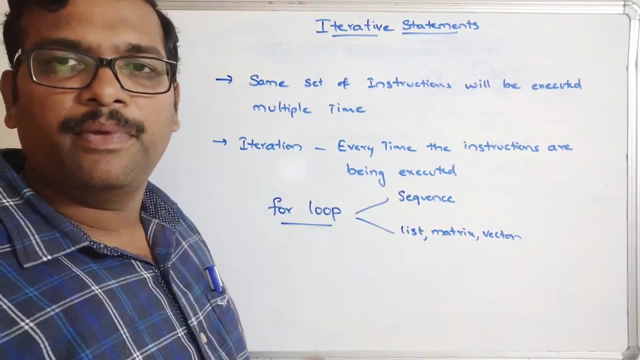 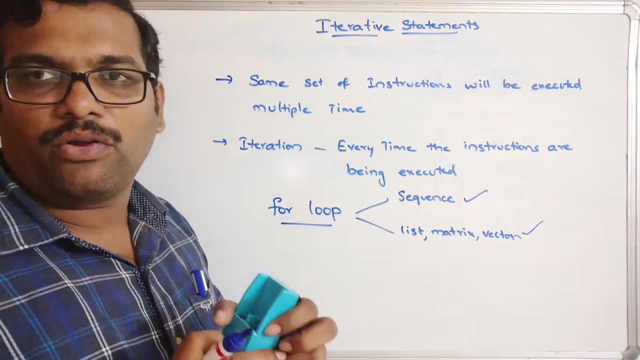 sequence. Now I will show you the syntax of this for loop in R programming here, and let us move to the R studio and I will implement a small program Demonstrating all these cases by using a sequence list, matrix and vector. So here the for loop will. 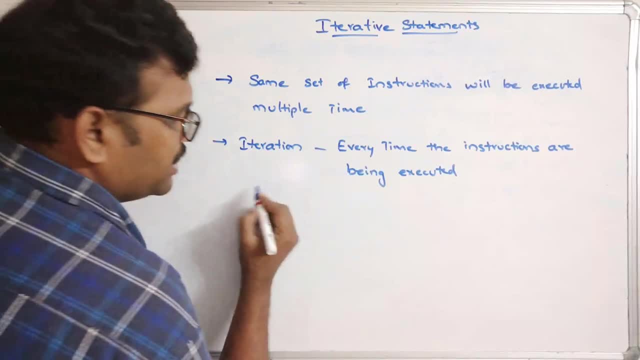 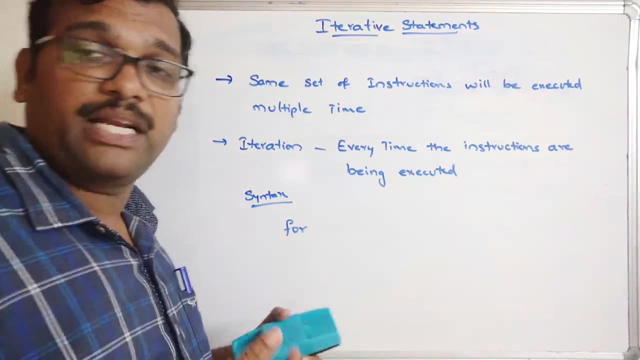 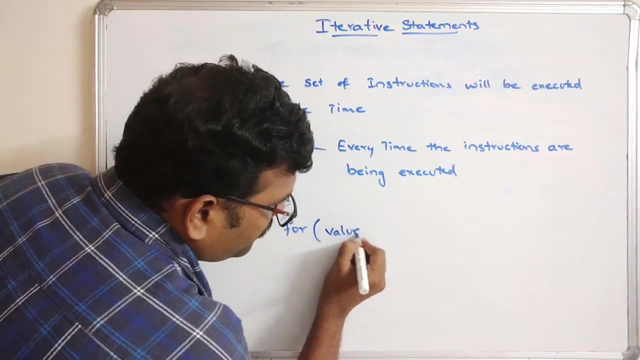 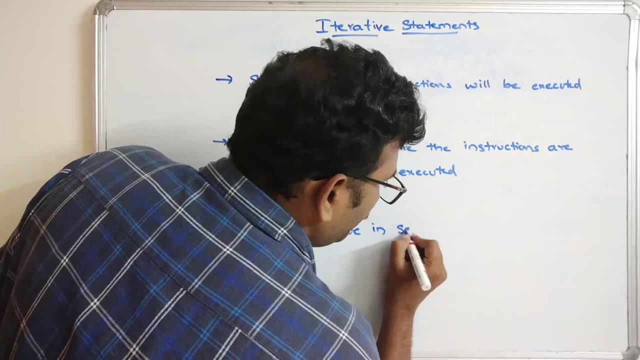 take multiple parameters. So the syntax for for loop. So use a keyword called for keyword. so keyword means a reserved word For open parentheses. give the value. give the value. use a an operator called in membership operator in. you can view here the 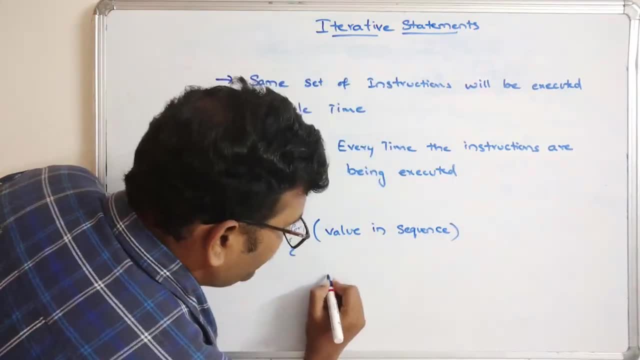 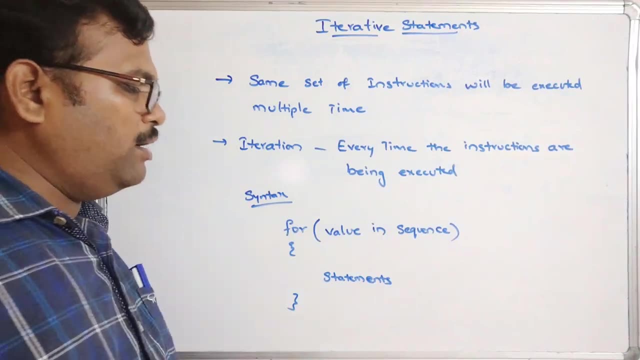 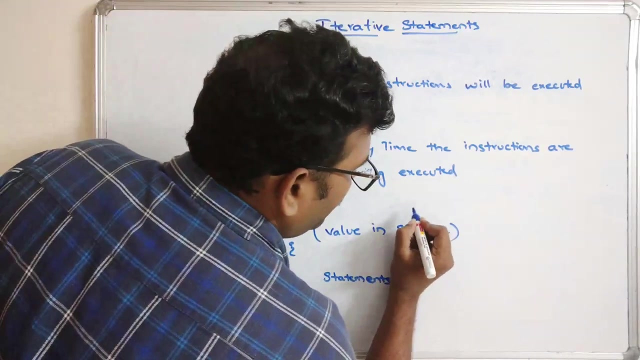 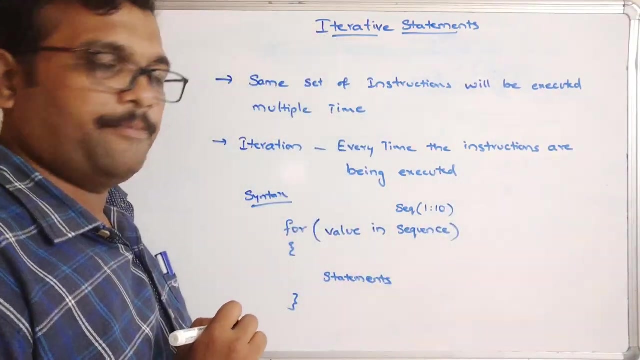 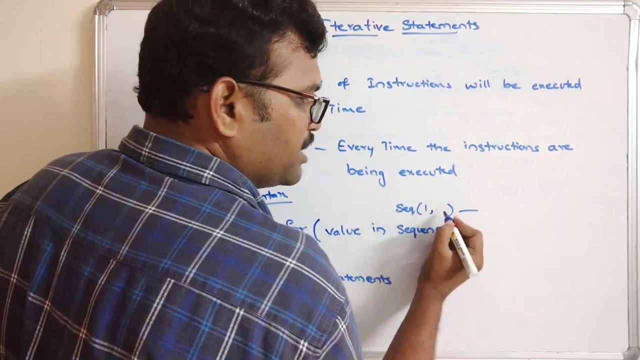 sequence, sequence, and here we need to write the statements statement. so this is a one syntax, one way of implementing the form, right. so here the sequence can be written as a sequence of one to ten, for example. okay, once of ten, okay, sequence of one to ten comma. so this implies: let a sex, a small value, let us. 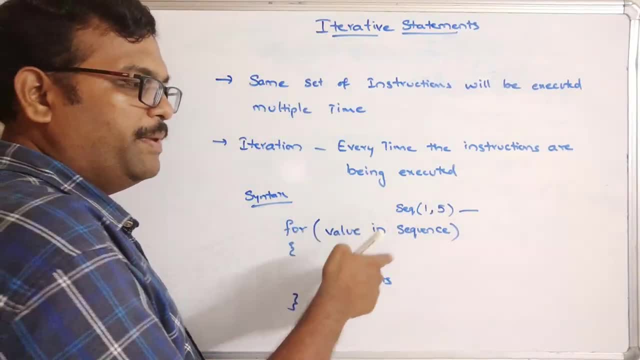 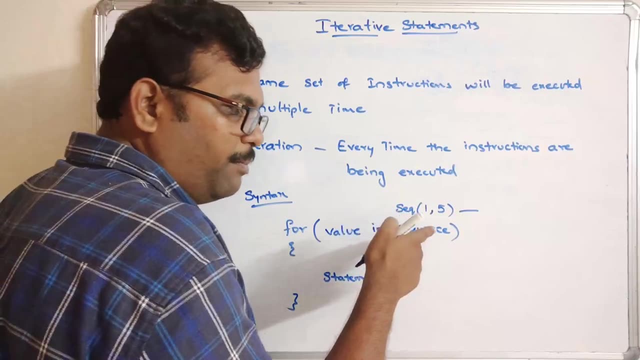 take one to five, so this value will be repeated. okay, I mean the value. if the value is available in this sequence, then only the statement will be get executed. that means the sequence one so, and then one first and five a, and then here we must accept anче order. on the syntax. that means the sequence one to ten. 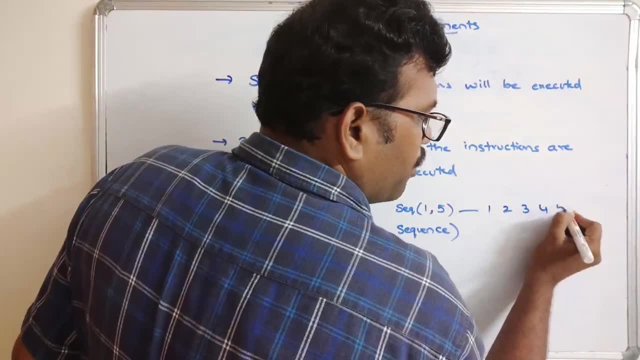 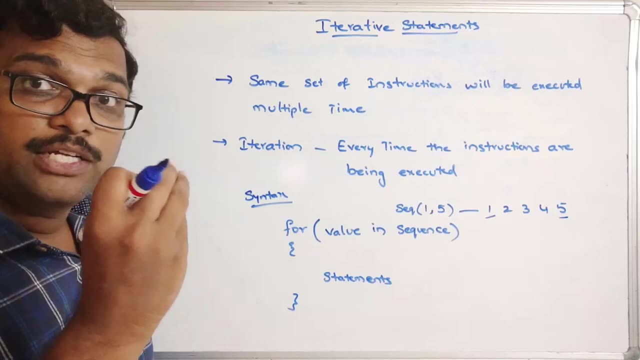 2, 5 means 1,, 2,, 3,, 4 and 5.. So from the first element onwards, from last element. So here we are having some 5.. So there will be a 5 possible iterations. Okay, There will be a 5 possible. 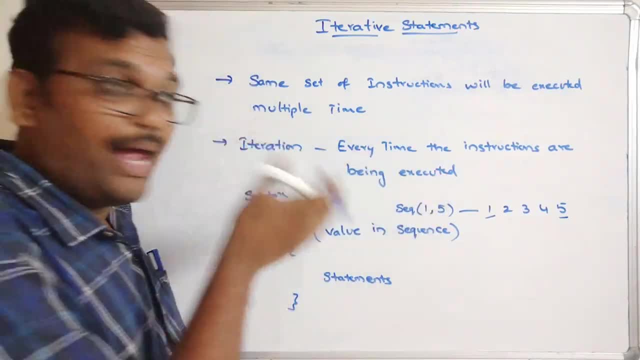 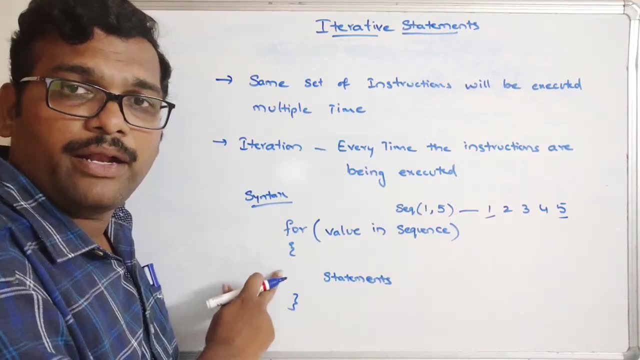 iterations if the value is available in this sequence. If the value is not available in this sequence, the control will never enter into the loop. Okay, The control will never enter into the loop, Only if the value is available in this sequence. Here sequence is 1, 2, 5.. So 1, 2,. 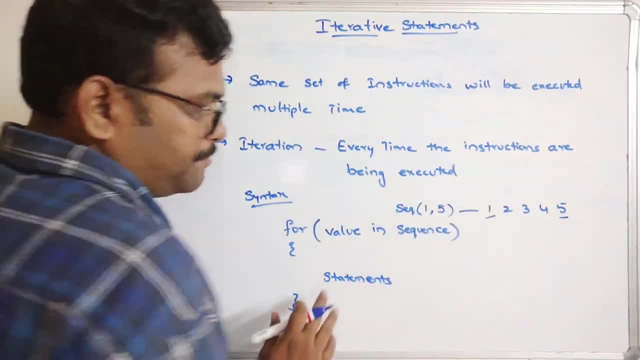 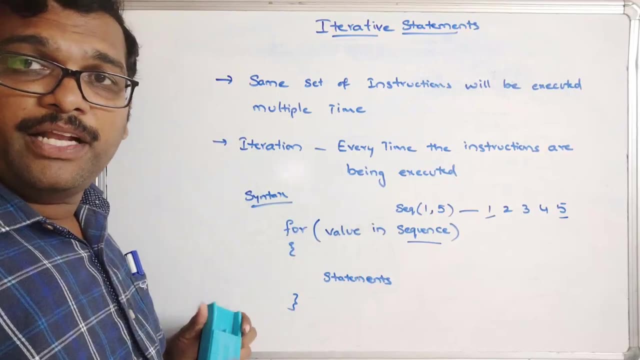 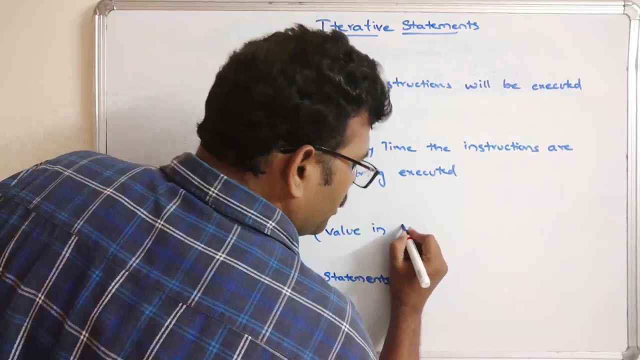 3,, 4 and 5.. Okay, So this is how we can implement the for loop by using this sequence. Another way of implementation is by using a list or vector or a matrix. So instead of writing here the sequence, we can write here the list or a vector or a matrix. 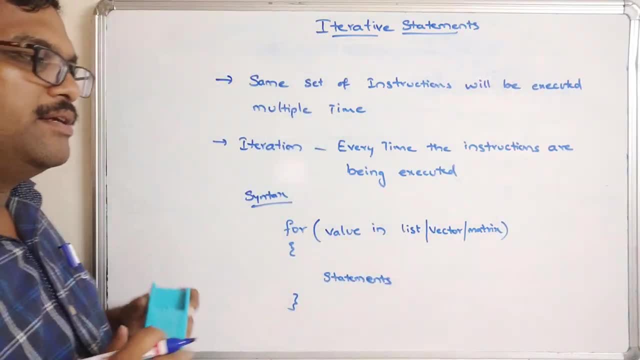 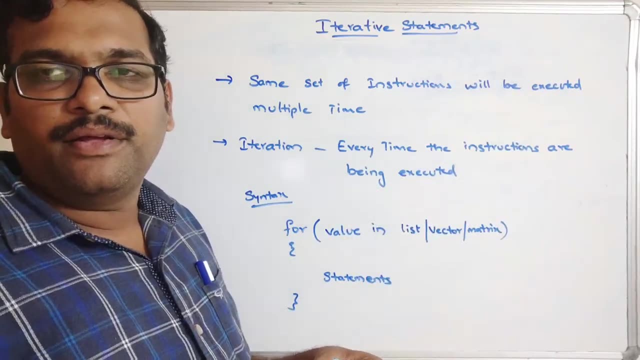 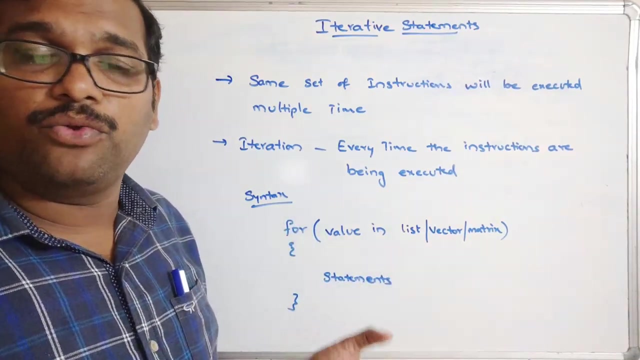 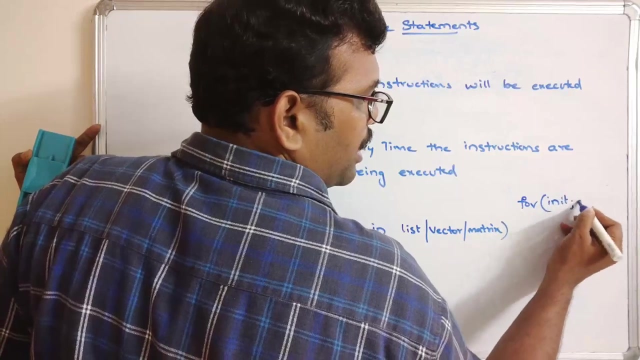 A matrix. So obviously it will be starting with the starting element and it will end with the last element, Right? So in such a way the for loop will be get executed. So in other programming languages we are going to use a syntax like for example in C for initialization condition. 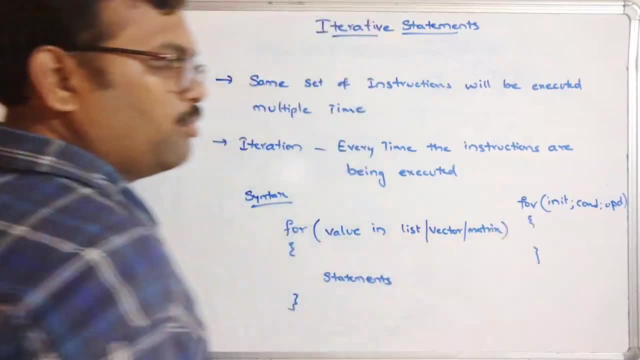 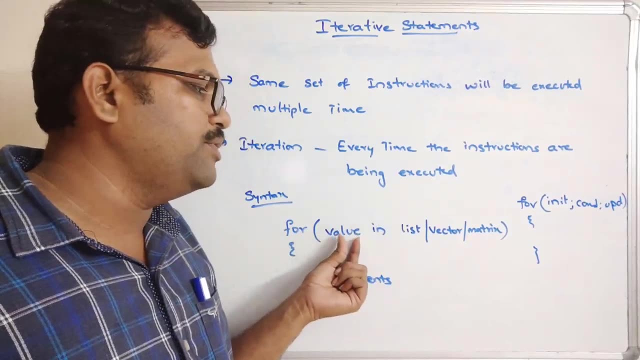 updation, So like that. we have to use a for loop, But here we are using the membership operator. We are using some value or expression and it will search whether this value is available in this particular sequence or the data structure And if. 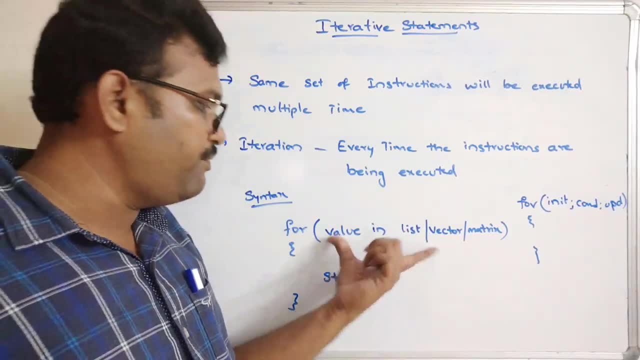 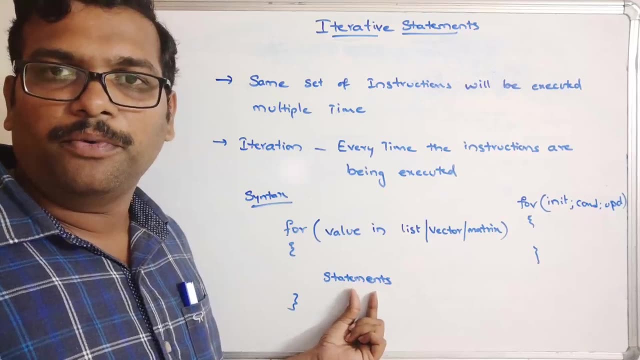 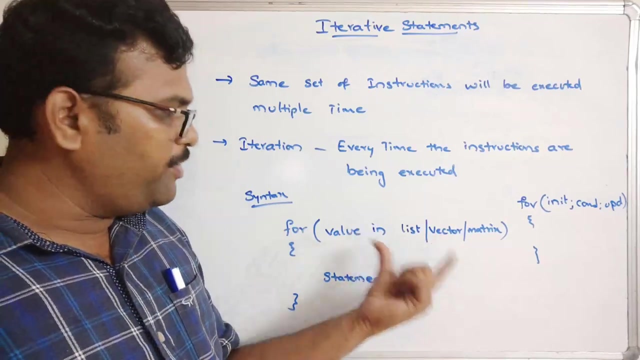 it is, then the following statements will be getting executed: So if this becomes false, automatically the condition- I mean the control- will never enter into the loop. So automatically it will skip from the loop. So at finite number of steps, obviously, the value. 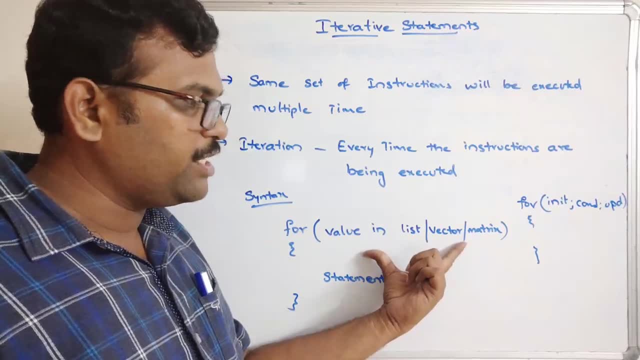 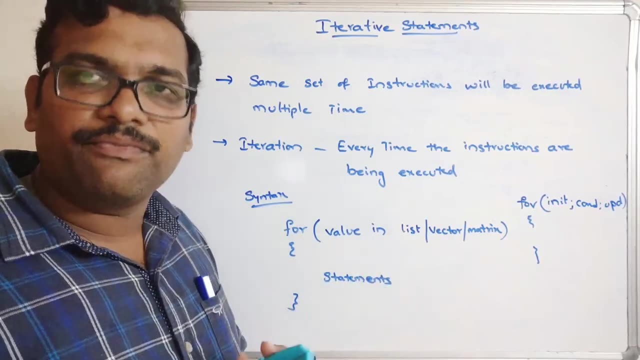 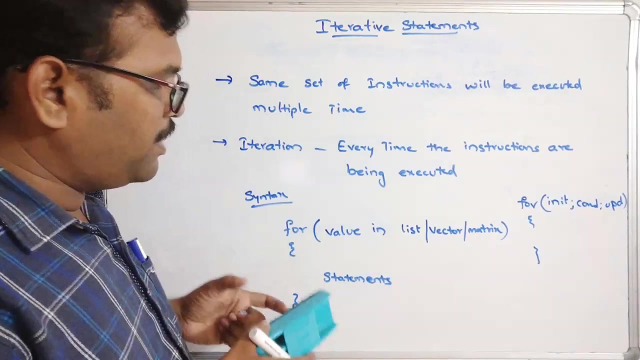 should be false. I mean, this particular section will become a false Right. So if it doesn't become false automatically, the loop will be infinite. The same set of statements will be repeated infinitely, Right? So these are the syntax for implementing the for loop using a sequence or: 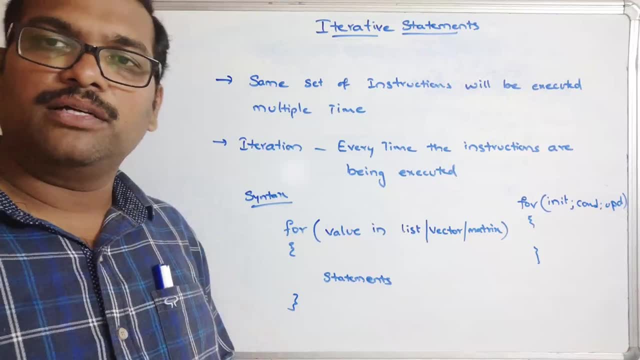 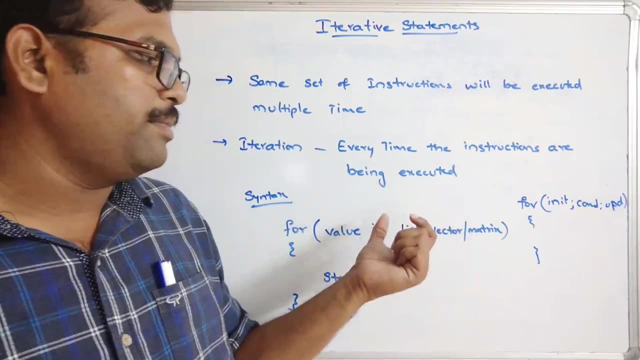 these data structures. And now let us move on to the R studio and I'll demonstrate each and every case. So, implementing sequence, implementing with the vector, implementing with the for implementing with a list, implementing with a matrix. So let us move on to the system. 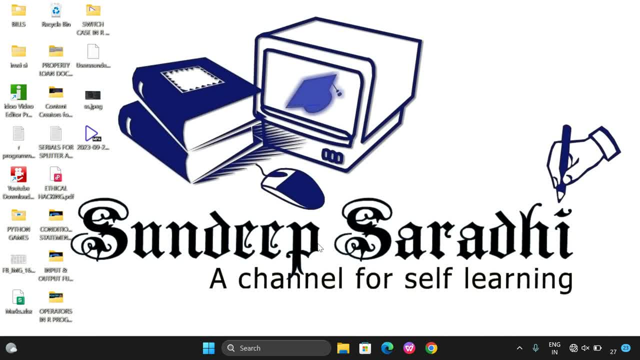 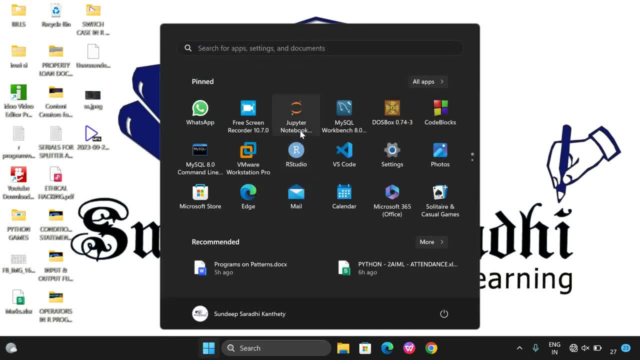 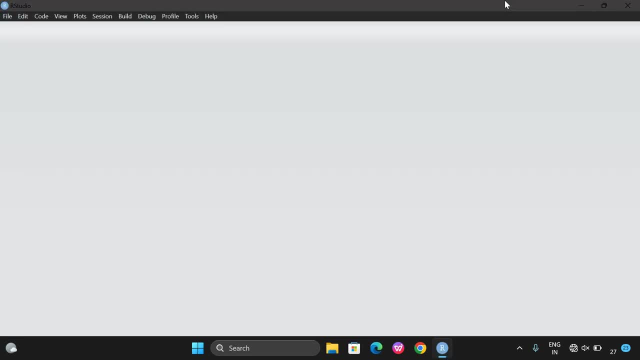 Hello friends. So just now we have seen the syntax of for loop, So implementing using sequence, and the data structures. Now we will see the direct implementation of all those cases, So how we can implement the for loop using a sequence and list or vector or matrix. 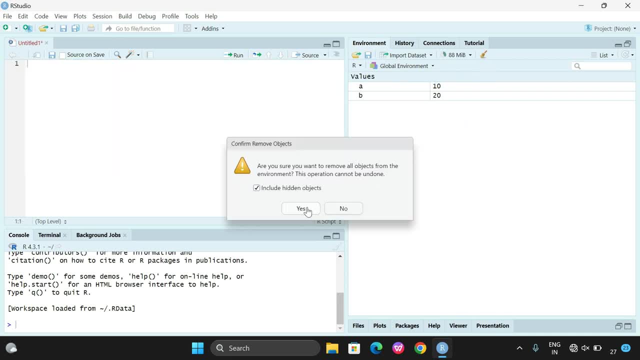 So let us take here I will clear all the remaining. I mean previous inputs and outputs. So now let us take one variable. So a is equal to. I will take. okay, let us give directly the for loop for: 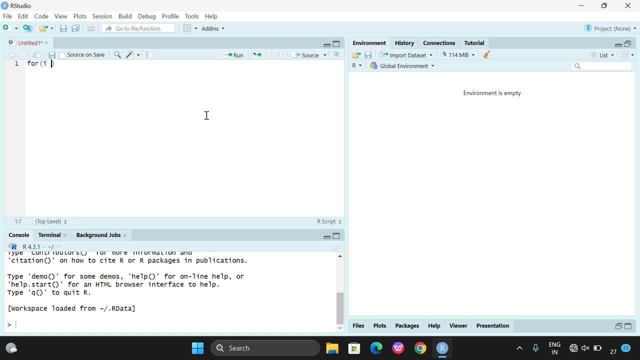 So let us take one variable or a value, So i in, and let us take the sequence, So sequence from 1 to 10,, 1 to 10.. And here I just want to print: i value, right, So we are. 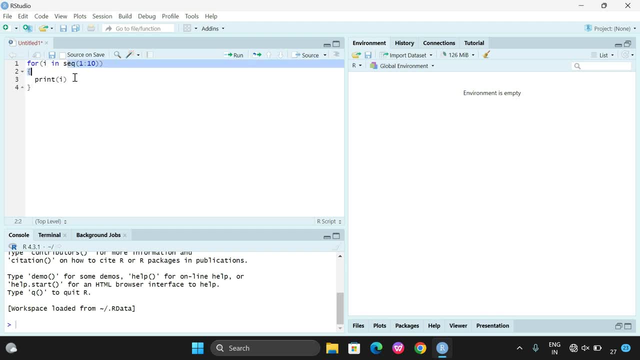 Just giving i value in this sequence. So i will be and this statement will be executed until i value is in this particular sequence, Okay, So, first of the sequence, 1 is to 10 means 1,, 2,, 3,, 4,, 5,, 6,, 7,, 8,, 9,, 10, right. 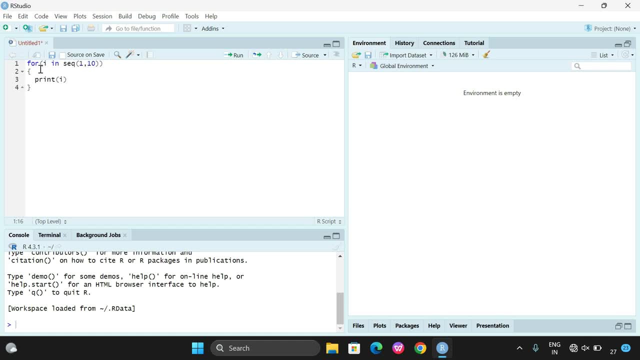 So until the i becomes 11.. So it will be: keep on true. So that is why this statement will be get executed. So once let us execute, See, you can, Let us give a small values, and now you can see 1,, 2,, 3,, 4, and 5, and if you give this one as a star and execute, so you will be getting see 5 stars, 5 different stars. 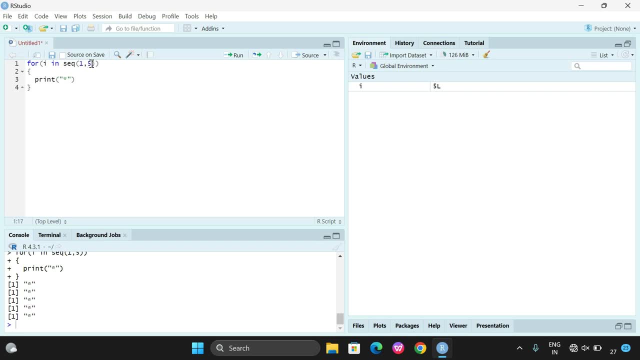 So this is just using a sequence, Okay, Just by sequence, right? So here in the sequence we are having a third parameter. That is a difference. So let us take some 10.. And And by is equal to two. 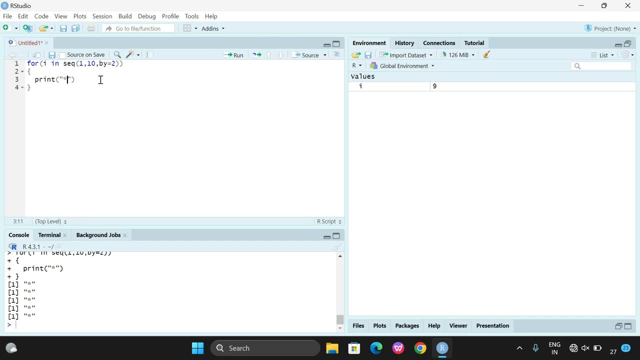 So that means it will take a difference of two. So let us print i value here. Let us print i value here, So you'll get 1, 3, 5, 7, 9.. So you can observe the difference between one number and another. number will be two. 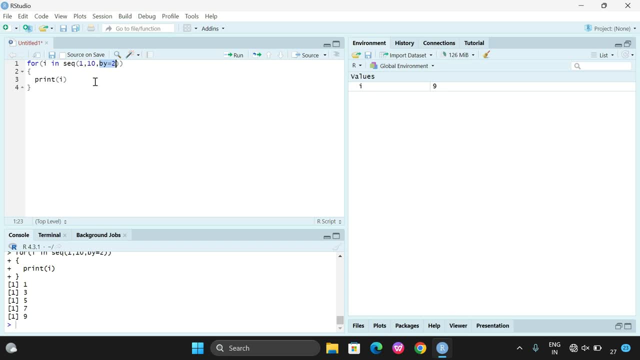 So the third parameter will give the difference over the upgradation updation right, The first number. it will start with one, So i value one in the first one And it will be printed And within the range right. 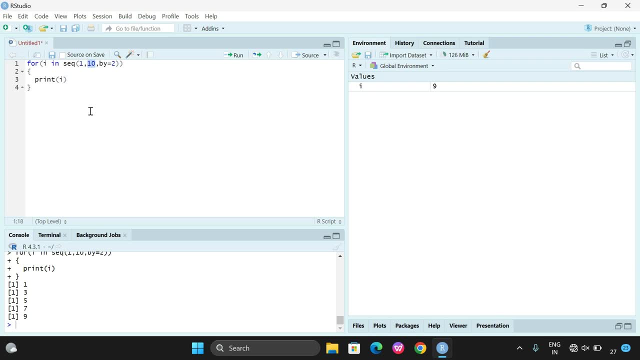 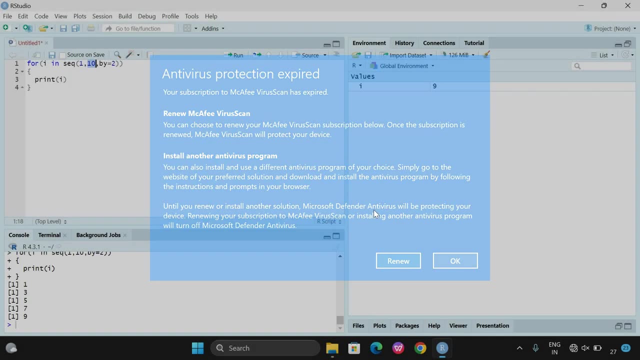 So here the 10 is a stop one right, So that will be treated as a termination. So whenever i becomes 10, it will be terminated. Okay, So similarly here also you can use any other updations. 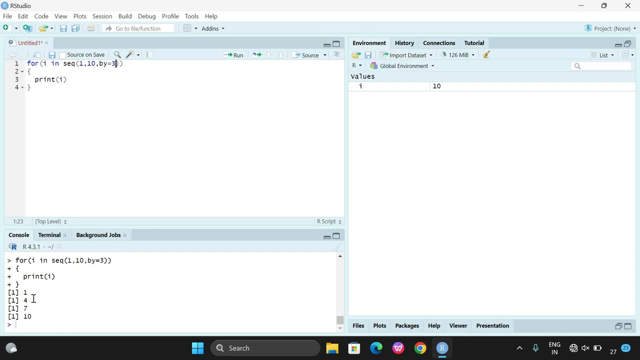 If I want to update with 3, so you can observe the difference over, the numbers will be 3.. So 1 and with a difference of 3,, 4,, 4 with a difference of 3,, 7 with a difference of 3, 10.. 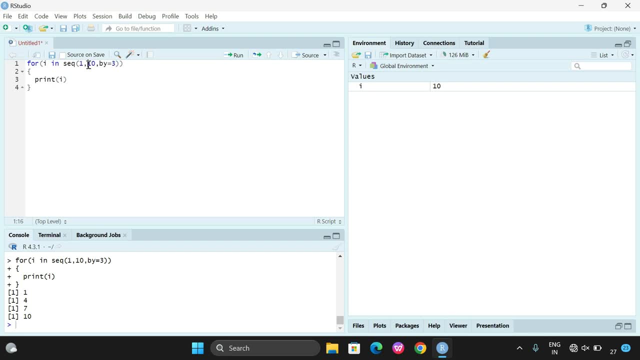 So it will stop at 7.. 10, because we are giving the stop as a 10, right. So first the sequence of values will be taken, And until the sequence of values, this particular statement will be get executed right. 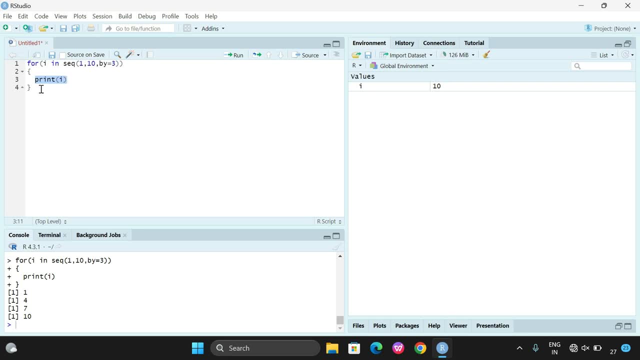 So this is an example for a sequence. sequence. Now let us check with the list. Sorry, a vector First. let us take a vector. So b is equal to, so vector can be initialized as a c of. I'll take 10,, 20,, 30,, 40,, 50. 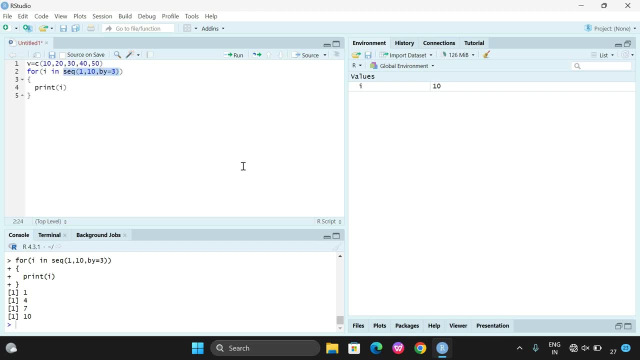 And here I can give it as a v right: I in v. So I will be starting with the value 10, and it will terminate at whenever i becomes a 50. So you can observe. So all the elements will be get printed. 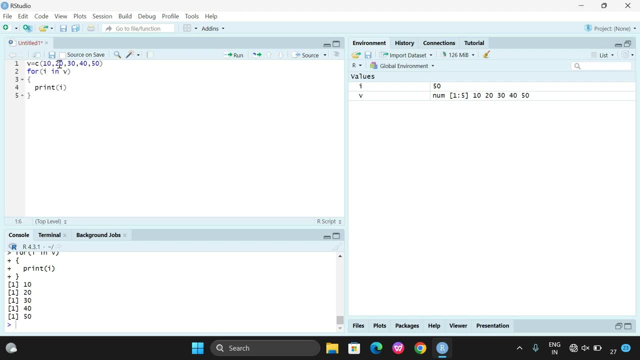 So I will be 10 in the first iteration. In the second iteration I will be 20.. In the third iteration I will be 30.. In the fourth iteration it will be 40.. In the fifth iteration it will be 50.. 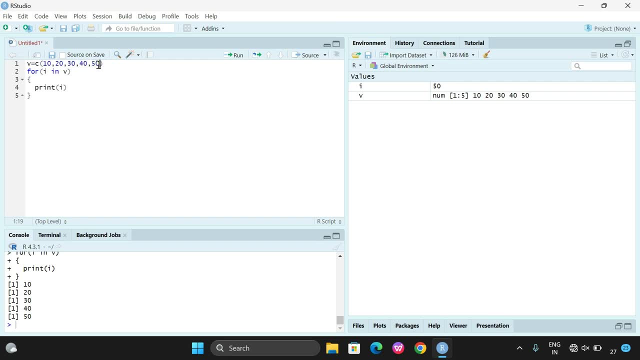 So whenever i reaches to the last of the element, last element of the vector, immediately the control will come out from the loop. So until it will repeat. So, for example, if you want to print any other, so star. 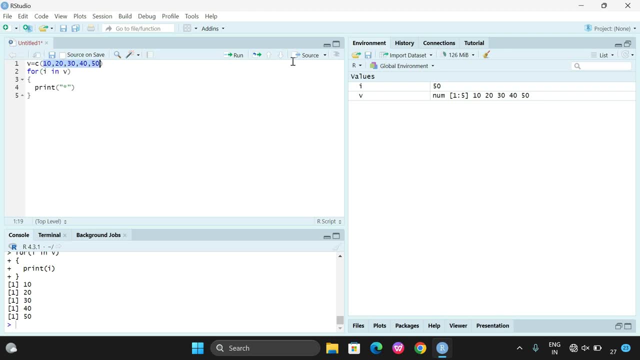 So how many elements are there? So total five elements are there, So five iterations will be repeated. You can observe: Five stars will be here, Five repetitions will be there. Okay, And also you can give any other versions. 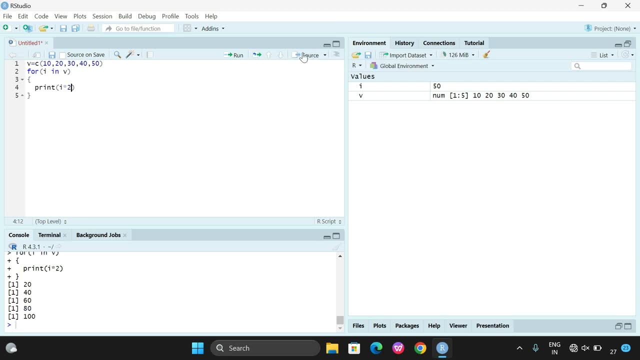 Okay, Any other expressions, I into 2.. So, if you observe, I into 2,, 10 into 2,, 20 into 2,, 30 into 2,, 40 into 2, and 50 into 2.. 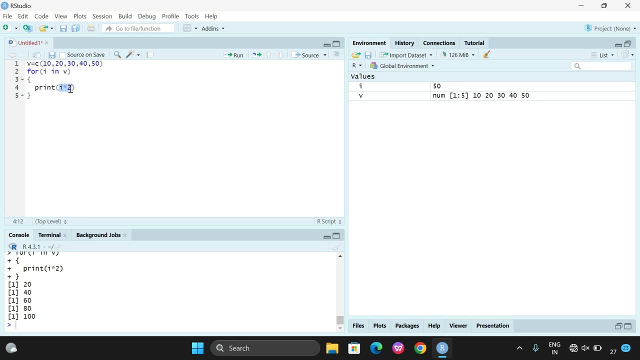 So, like that, we can give any other expressions. So, but until the i value reaches to the last element of the vector, this particular instruction will be keep on executing. Okay, Now see. this next one is a list. If I take it as a list, we know that l is equal to list function. list of. 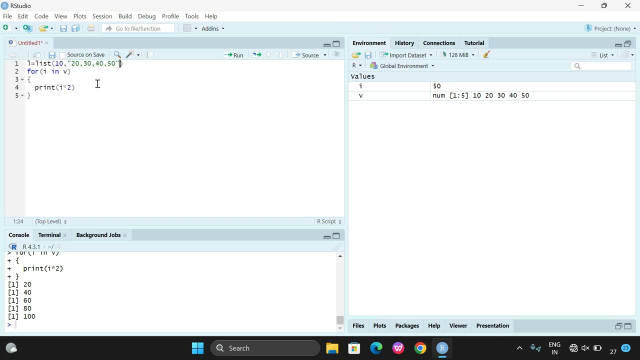 So let us take all the different data types. We can take a different data type, So I will take it as a ABC ABC And I will also take some 90.5 float value. Okay, And let us check. i in l. 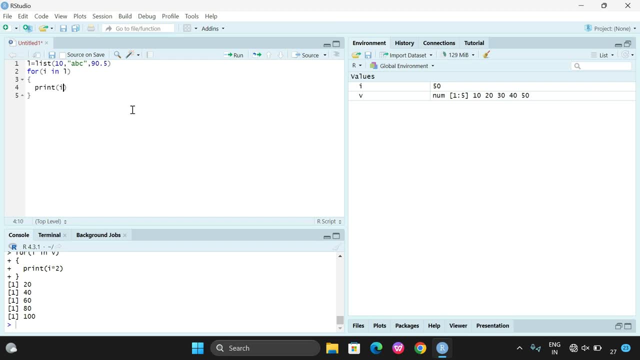 i in l, And here you can see print i. Obviously All the complete elements will be get printed, So 10, a, b, c and 90.5, everything will be get printed. So here, also similar to a vector, it will start with the starting element. 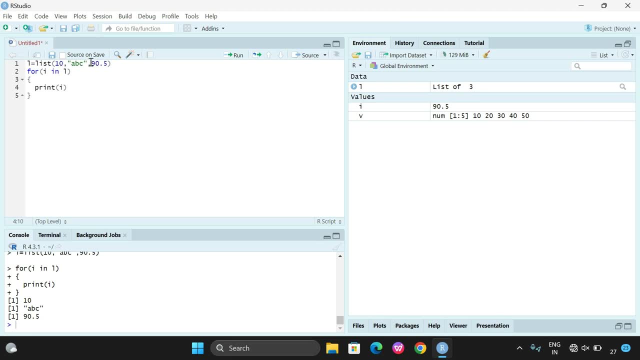 Okay, And it will end with the last element Right, Directly. it will iterate. So here, three elements are there, So this statement will be repeated three times. This statement will be repeated three times, So if you don't want to use these type of data structures, 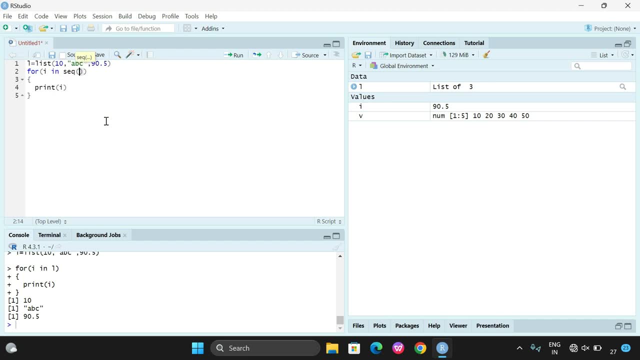 Simply, You can use a range That is called a sequence. So how many iterations? So the same set of statements should be iterated for five times, or 10 times. So give here 10. So 1 to 10.. 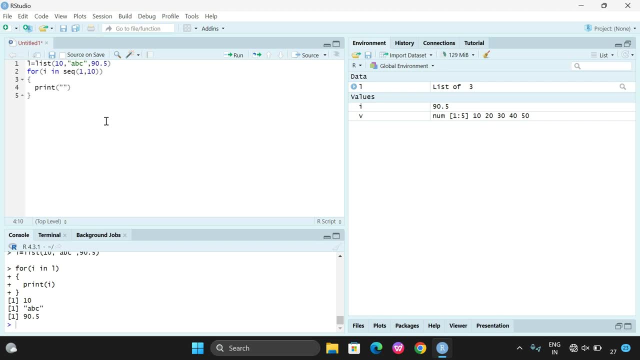 Right, And here give the value like Sandeep Right. So execute So 10 times. the instructions will be being executed 10 times. Okay, So the next one is a matrix. So we have seen the vector. 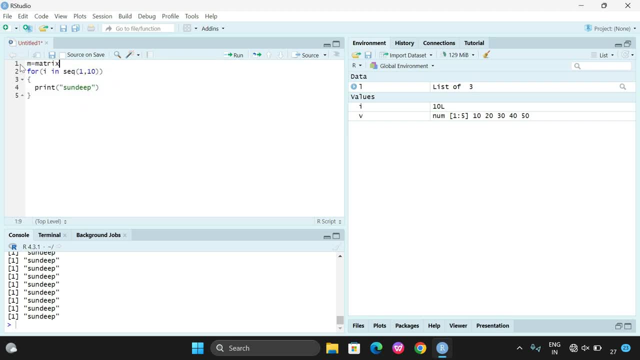 List Sequence. And now we will see the matrix. So we know that matrix can be created with the help of a matrix command and matrix function. So the first parameter will be the vector of values. I will take some four values. 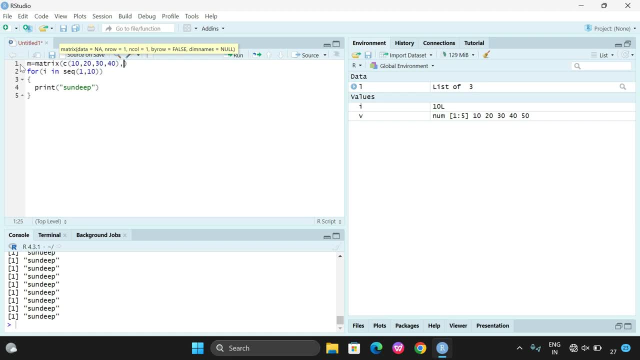 10,, 20,, 30, and 40.. And after that we need to give a number of rows and number of columns. N rows is equal to 2.. N columns is equal to 2.. Right, And instead of here sequence list or vector, we can simply pass M. 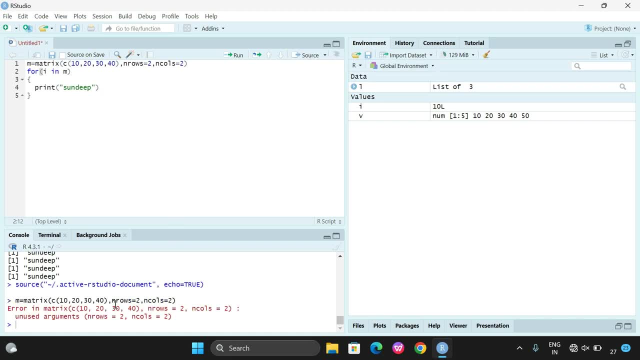 M is nothing but a matrix. M is nothing but a matrix. See, Yeah, Sorry, And yeah, N row and N column. Yes, So you got the same 10,, 20,, 30,, 40. Okay, 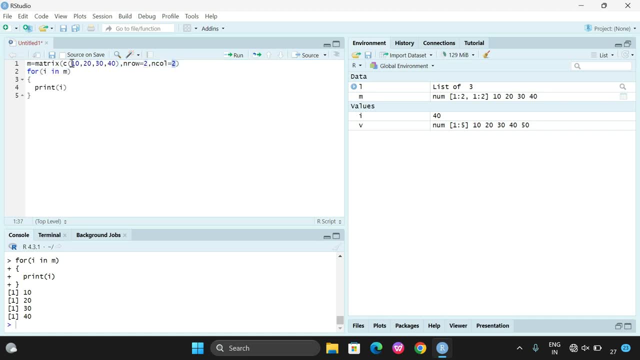 So N row, N column. So we are giving two rows and two columns And here we are giving some four different values And in all the cases we are printing some I, Or else you can print some any other character.